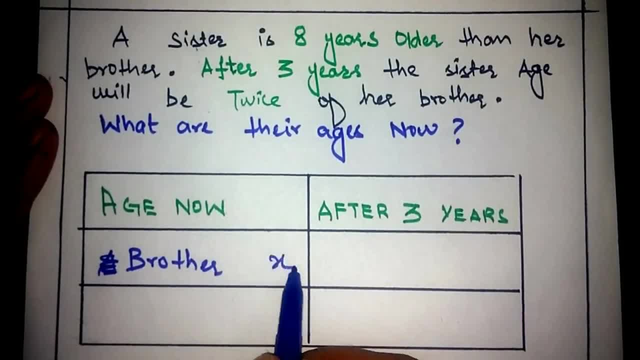 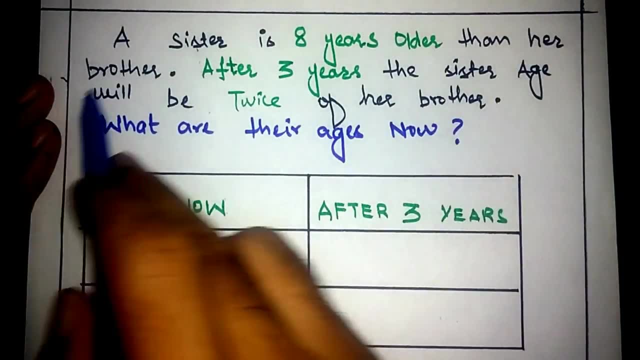 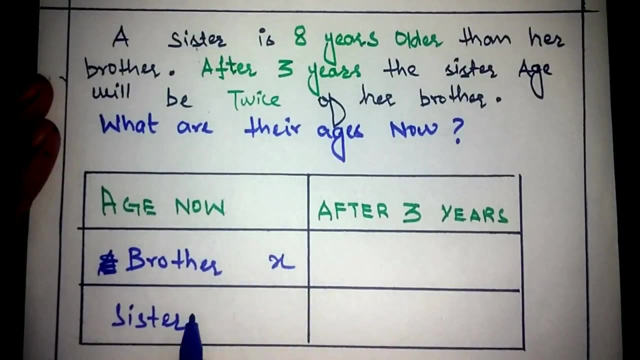 brother is- let's suppose we will denote it from X and the age of the sister is here you can see a sister is eight year older than her brother, so sister is eight year older. if the age of the brother is X, then the age of the sister will be X. 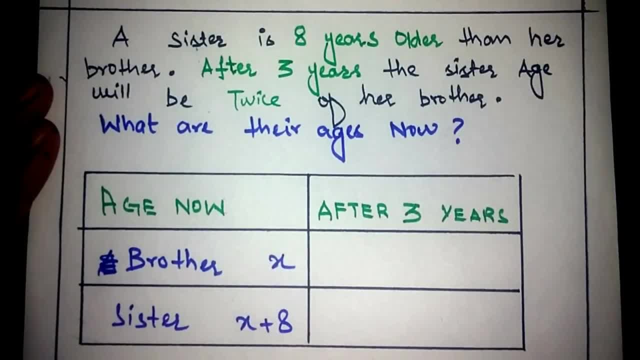 plus eight now write the ages after three years. so how can we write the ages after three years? if now it is X, after three years it will be X plus three, and if now the age of the sister is X plus eight, after three years the age of the 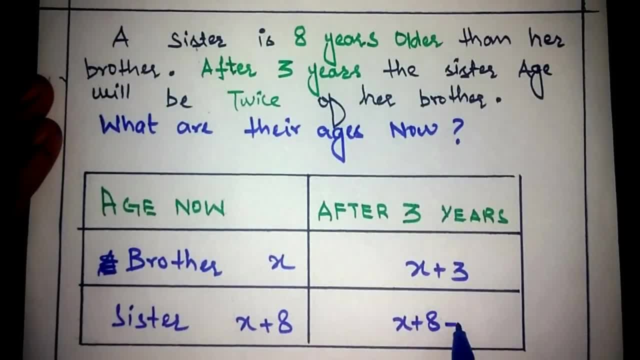 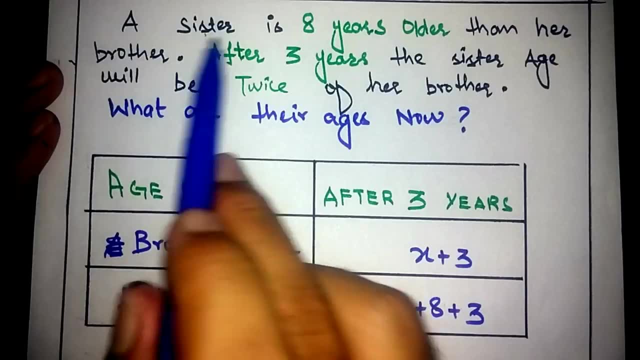 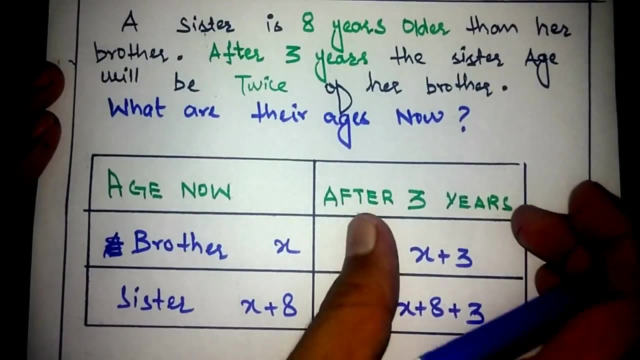 sister will be X plus eight plus three. so now we have made the equation for the present ages and for the ages after three years. the next step is after three years, the sister age will be twice of her brother. so after three years the sister age is this and the brother age 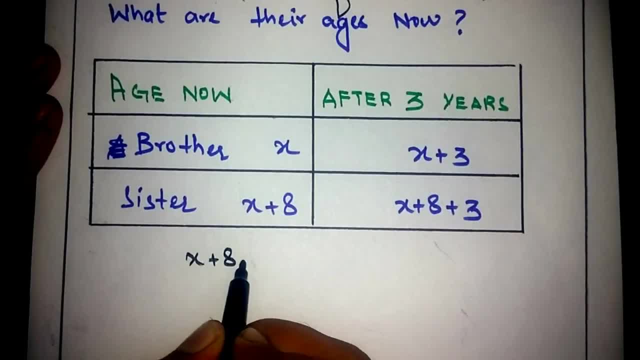 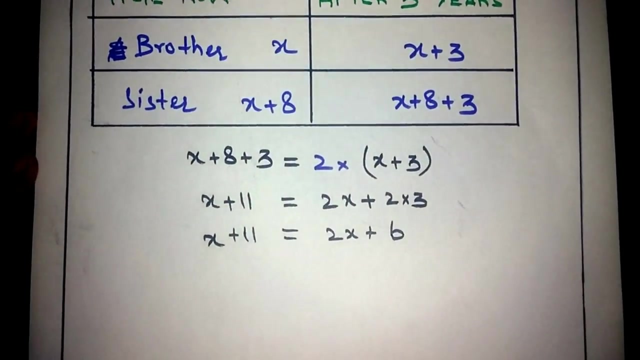 is this. so this will be twice of this. here, you can see, this is twice of this. the sister age after three years is twice of her brother. now the rest is very simple. just solve for the value of X. here you can see this: X is plus here. so after coming to this side, it will become: 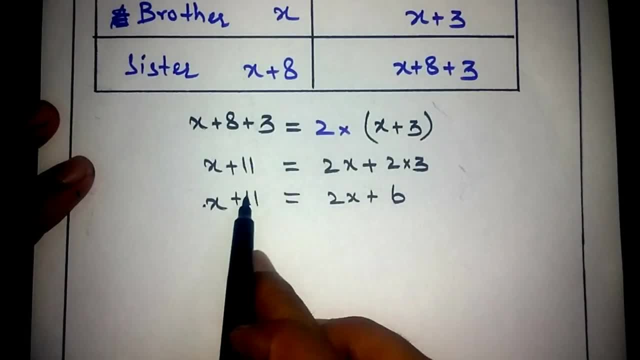 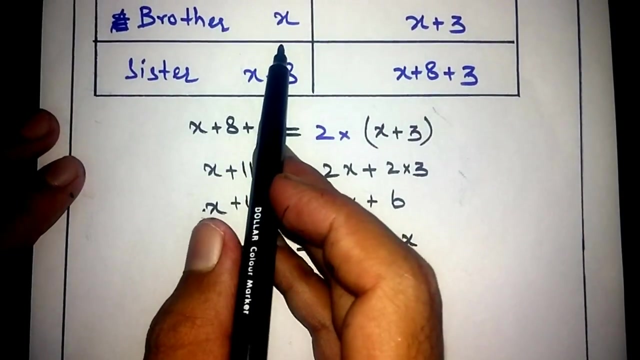 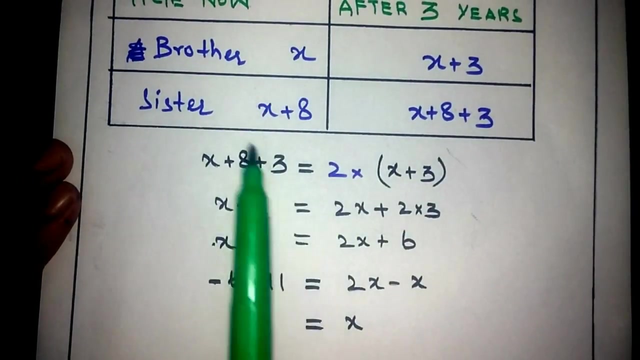 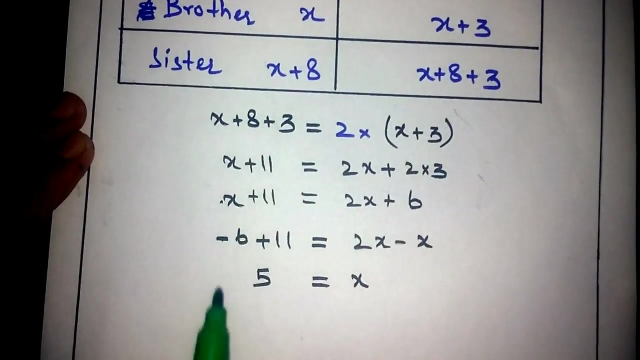 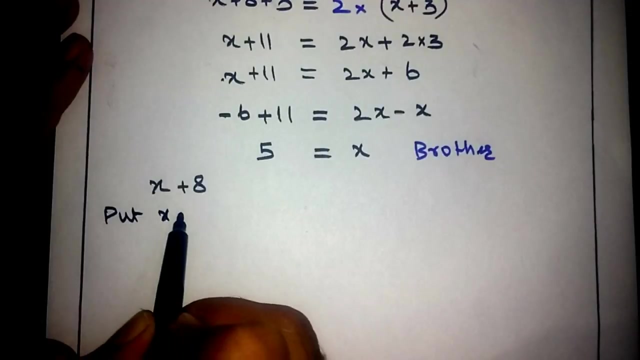 minus X here and here this six is plus. so come to this side of equal, it will become minus six. you Ni역a its value. okay, so the orders will come down. this says that the age of Return a row will take. this value is minus 6th of x is equal to the age of. 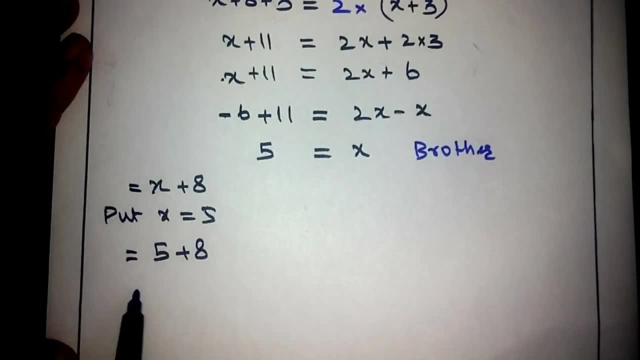 the sister. so let's do it. Put: X is equal to 5 if it is equal 2- 30. so the age of the brother is X is equal to 5, and the age of the sister is X plus 8, and which is is equal to 30. 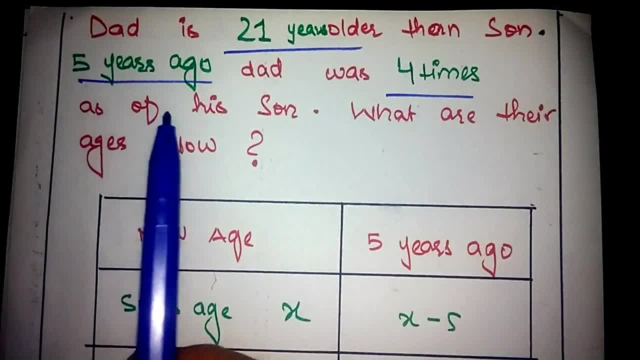 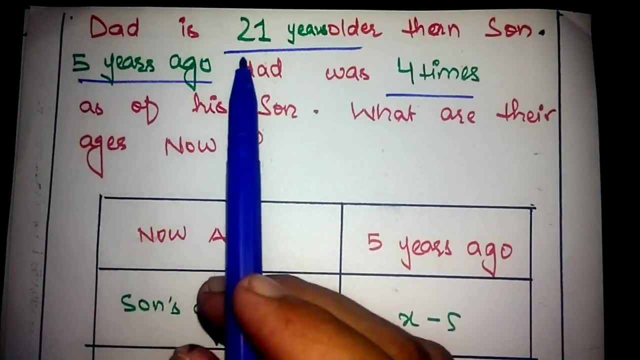 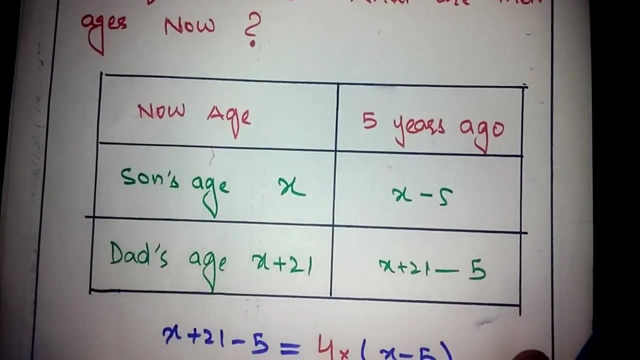 this is the next age problem: year older than his son. five year ago that was four times age of his son. what are their ages now? so important points are: 21 year older five year ago, four times. the next step in this type of question is to draw a table with six blocks, two columns, three rows and here write the now ages for. 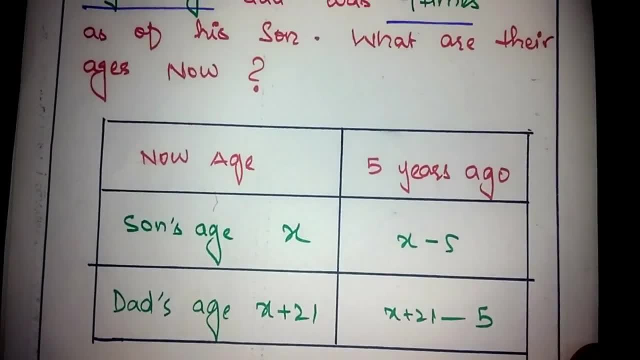 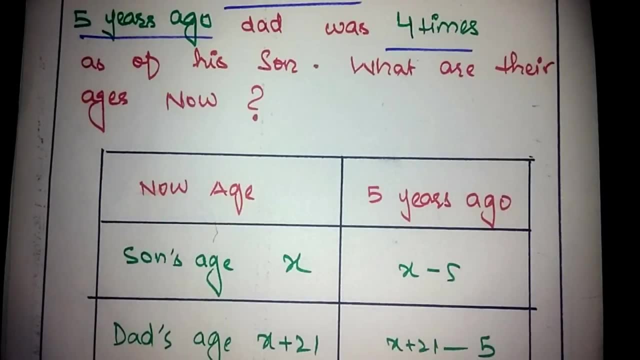 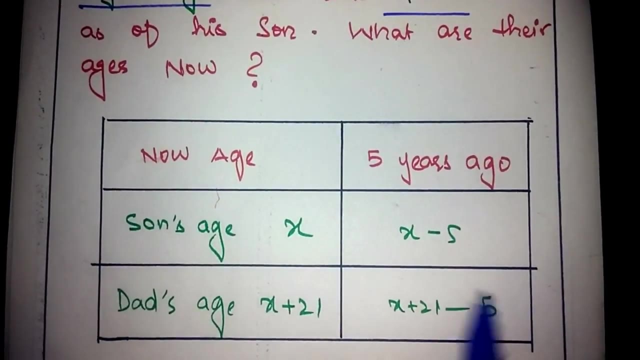 present ages and here write the ages which is given. here you can see five very ghosts. so right here, five year ago- the next in the question- it's dead- was 21 year older than his son. so if the age of the son is x, then the age of the dead will be x plus 21, because dad is 21 year older than his son. 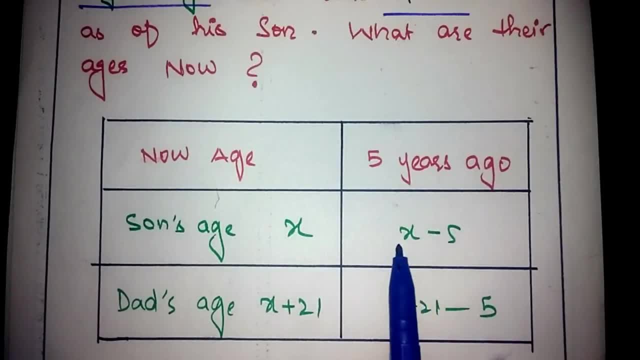 so five year ago means in the previous five year. for the ago time we write minus. so if the age of the sun now is x, five year ago it was x minus five. if the age of the dead now is x plus 21, five year ago it was x plus 21 minus five. 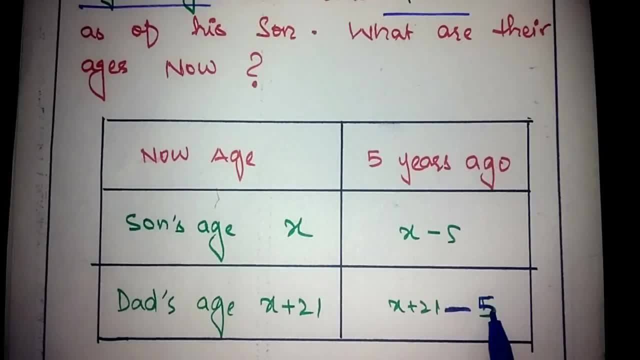 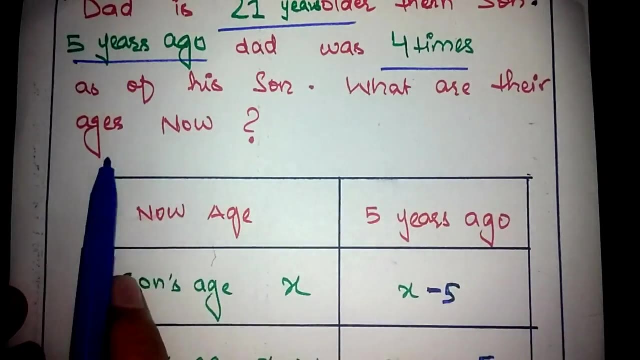 here you can see this minus five is for previous time. so we have equation for the present ages and also the equation for the ages are before five years and next in the question it says five year ago it was four times edge of his son. what are their ages? 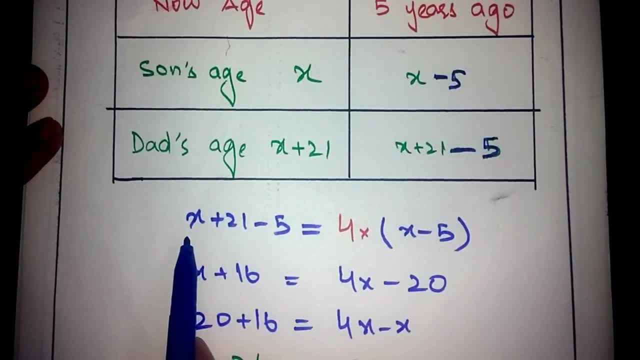 dead was four times as of his son. so five years ago. the age of the dead is this: and he was four times as of his son. this is the age of the date, five years ago, and this is the age of the sun, five variable. and that is four times as of his son, as of his son. so the next. 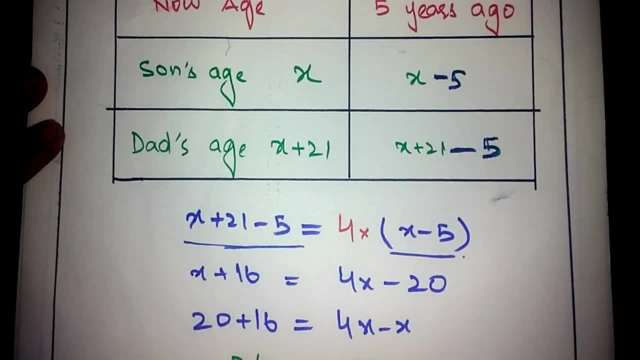 is very easy. just solve it for the value of x. and what is x? here you can see, x is the age of the sun. So if you find the value of x, it means that you have found the age of the sun, present age of the sun. 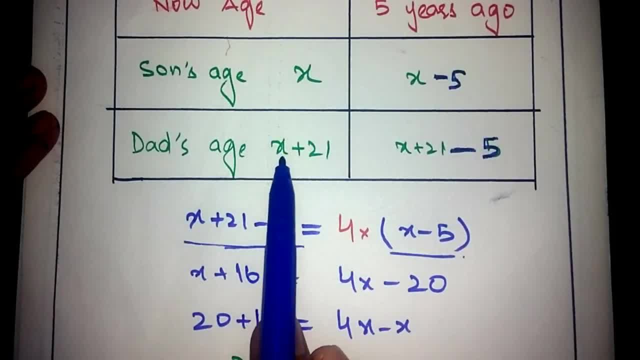 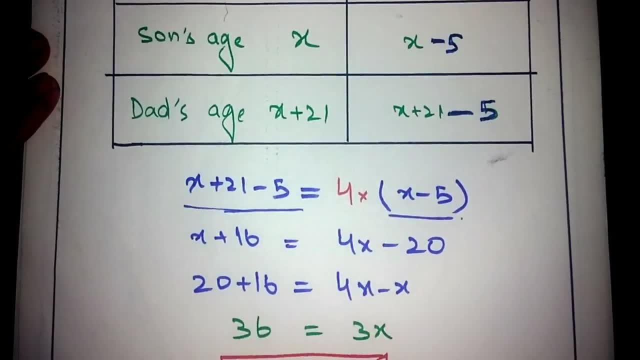 And what will be the present age of the dead? Put the value of x here and you will be with the age of the dead. So let's do it Here. you can see: 21 minus 5 is 16 and this 4 times x is 4x. 4 times 5 is 20 and minus.